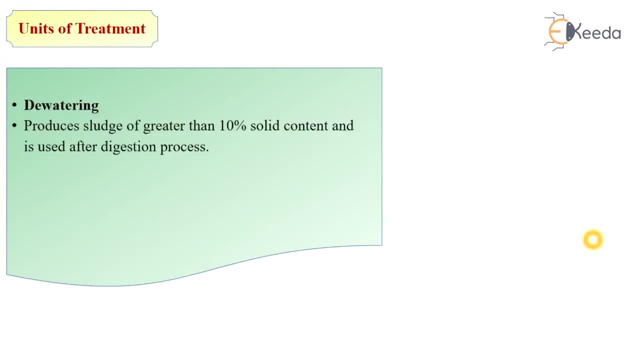 What is dewatering? It produce the sludge of greater than 10% solids content and is used after digestion. So dewatering means the reduction of water content in sludge and make it up to 10% of solid contents in that sludge. So after that we are applying the sludge onto the sludge. 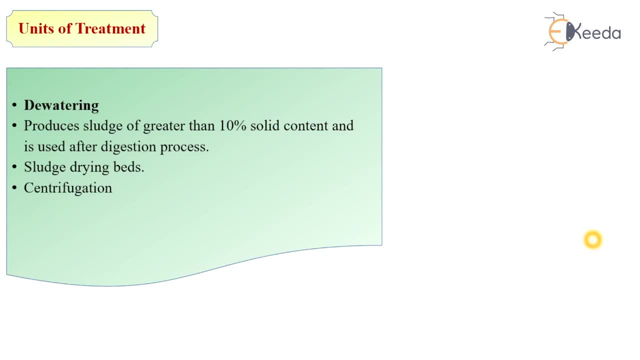 drying beds. Then centrifugation happens, takes place there, and mechanical methods by vacuum filtration also we are applying. So what is dewatering of sludge? The digestion process is done by the digester, by the machine which contains lots of water, which should. 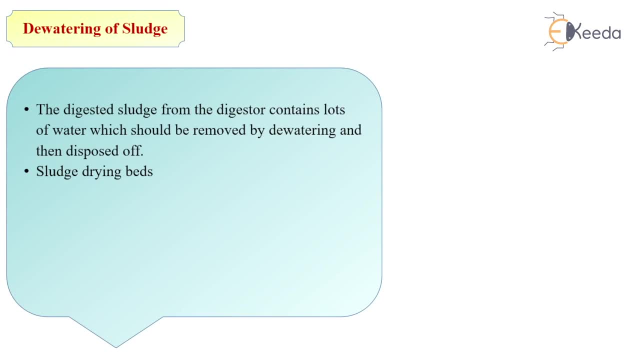 be removed by dewatering and then disposed of. So for that we are providing the sludge drying beds. So in mechanical methods, the dewatering, drying and disposal of sludge by the sludge drying beds, the drying of digested sludge on open beds of land or sludge drying. 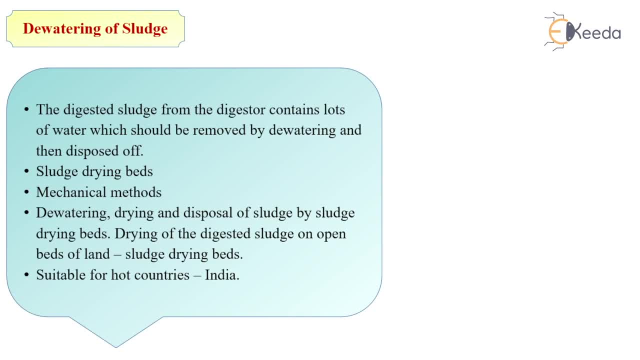 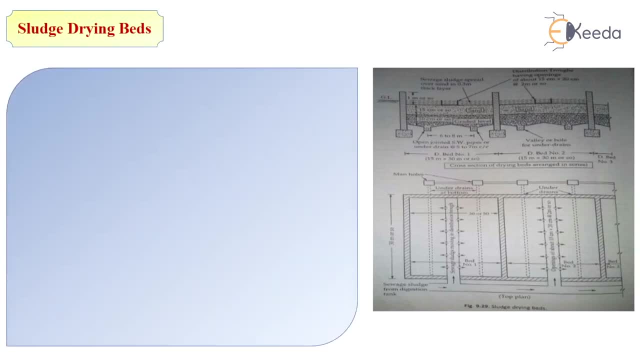 beds. It is suitable for hot countries like India. So, as you can see in this diagram, these are the sludge drying beds. There are number of units in that we are providing some media or material. So let's we see the construction of the sludge drying beds one by one. 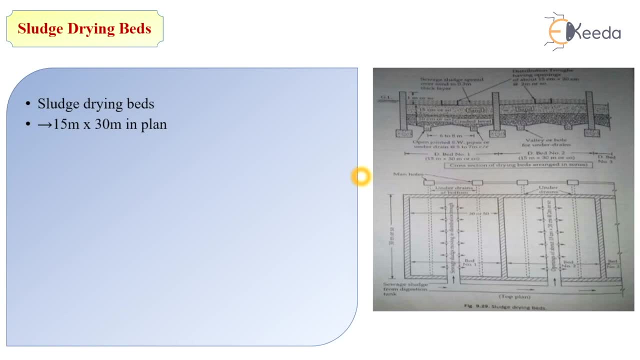 So sludge drying beds are of sizes of 15 by 30 meter in plan and 45 by 60 centimeter in depth. So depth of this sludge drying beds are usually kept as 45 to 60 centimeter. So area wise, it should be a 0.05 to 0.2 square meter per capita. 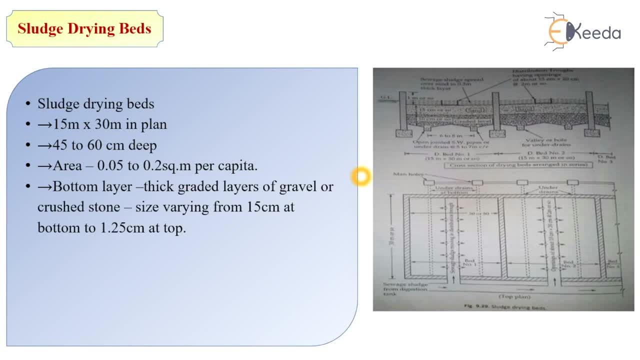 So per capita requirement for the sludge drying beds. the area of that is 0.05 to 0.2 square meter. The bottom layer is provided with thick threaded layer of gravels or crushed stones. The size of these gravels are varying from 15 centimeter at bottom and 1.2 centimeter at top. 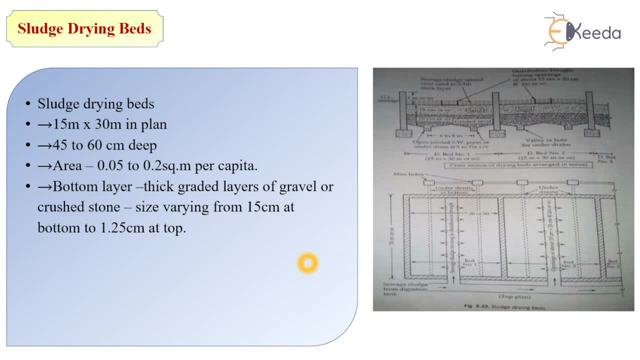 That means the bigger size particles are kept at bottom and smaller size gravels are kept on its top. The top layer consists of 10 to 15 centimeter thick coarse sand layer, So the bottom layer is provided with thick threaded layer of gravels or crushed stones. 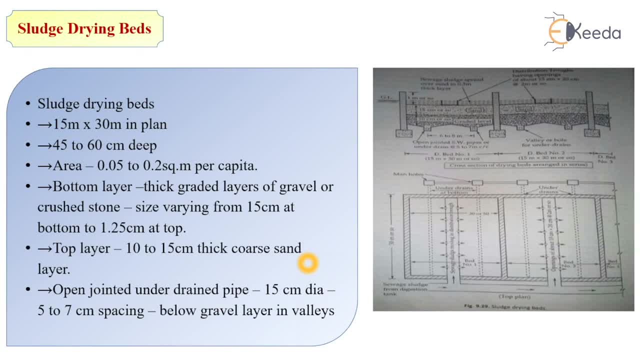 The bottom layer is consist of coarse aggregate and the top layer is consist of sand. Then the open jointed under drain pipe is provided there: 15 centimeter of diameter and 5 to 7 centimeter of spacing. So, as you can see in this slide, 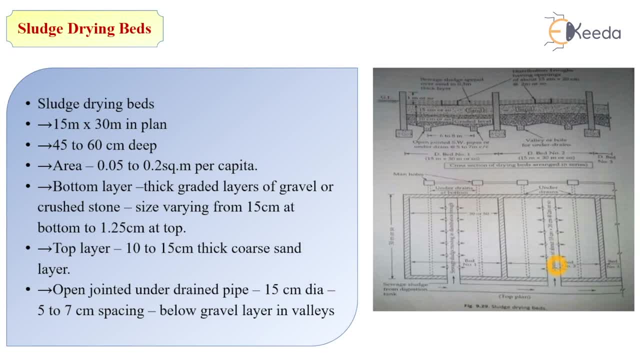 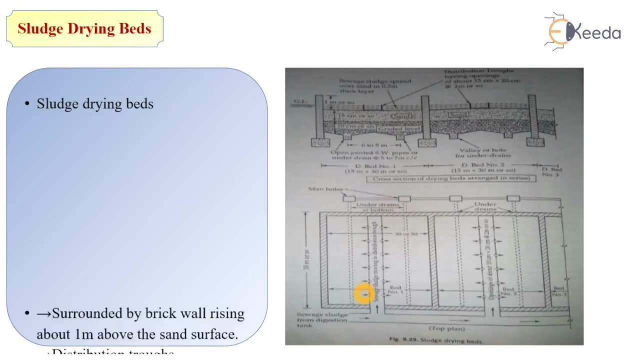 So, which is the under drainage pipe below the gravel layer in valley, So at the bottom layer of this gravel, we are providing the under drainage pipe, Under drainage system for collecting the water. Then the surrounded by brick wall rising about 1 meter above the sand surface is constructed. 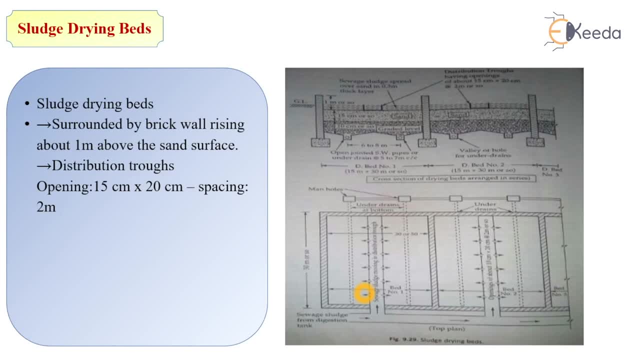 The distribution trough, the opening of 15 centimeter by 20 centimeter and spacing of 2 meter. the distributing trough should be provided Sea wet sludge from digestion tank is spread over the top of a depth of 20 to 30 centimeter. 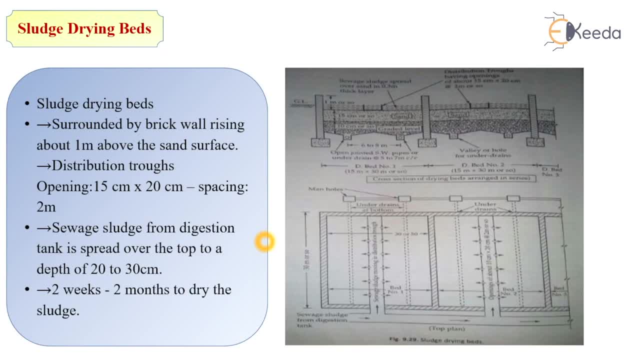 So it is remains constant or stable for 2 weeks to 2 months to dry the sludge. So this process will continue for the 2 months. So, again, this is long process. So, as you can see in this diagram, 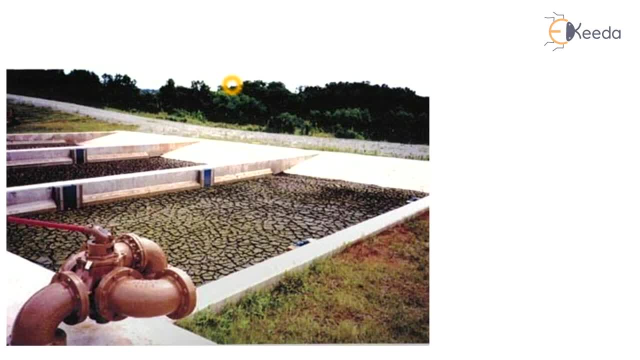 These are the sludge drying bed And which is suitable for hot temperature, hot conditions like in India. So the depth of this drying beds are approximately 45 to 60 centimeter, And we are providing the under drainage system for collecting the sludge, liquor or water from the bottom of this tank. 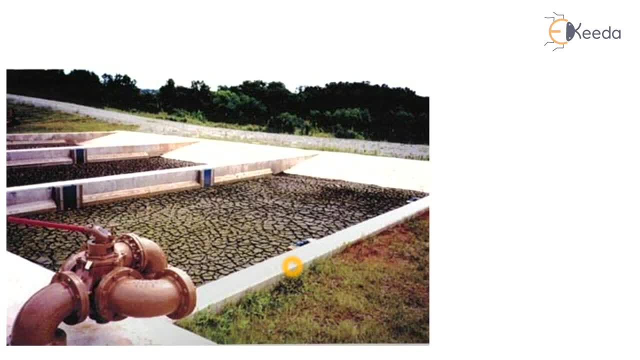 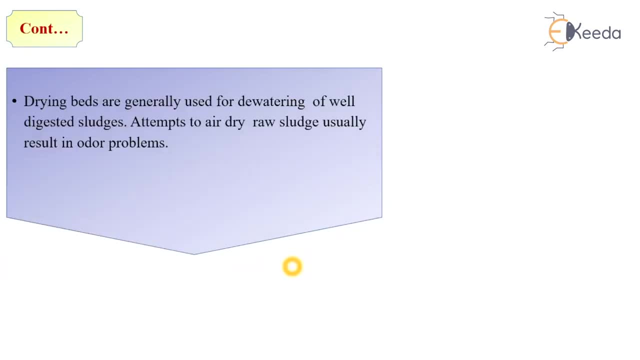 And this process is continue for minimum 2 months. So the drying beds are generally used to collect the sludge. So the drying beds are generally used to collect the sludge. So the drying beds are generally used for dewatering of well digested sludge. 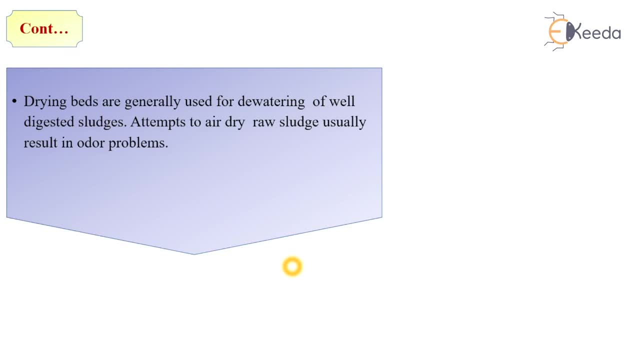 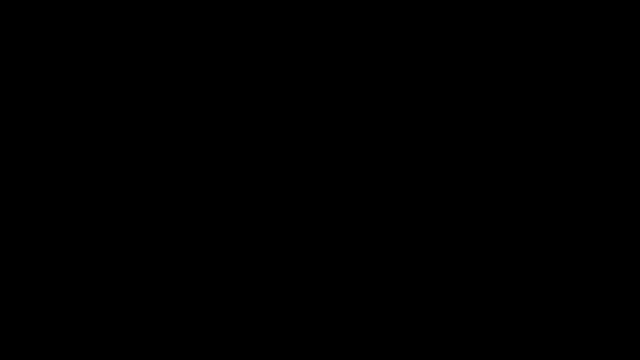 Attempts to air dry raw sludge usually results in odour problem. So sludge drying beds consist of perforated or open joint drainage pipe laid within the gravel base. Thank you, Thank you, Thank you.